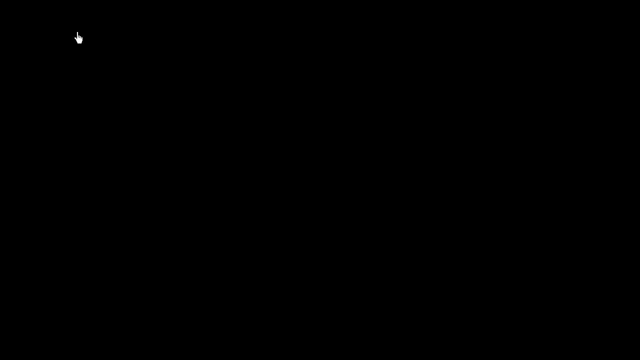 I will now do a proof, for which we credit the 12th century Indian mathematician, Bhaskara. So what we're going to do is we're going to start with a square. So let me see if I can draw a square. I'm going to draw it tilted, at a bit of an angle, just because I think. 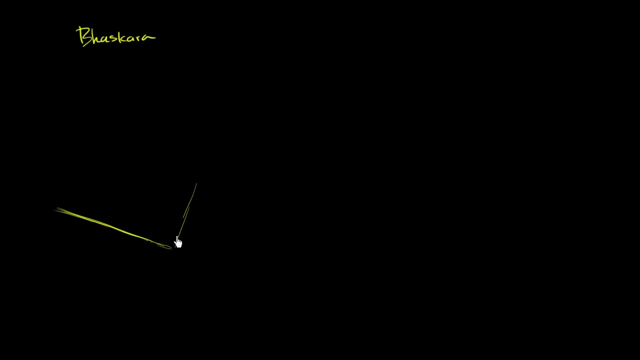 it'll make it a little bit easier on me. So let me do my best attempt at drawing something that reasonably looks like a square. Bear with me if it's not exactly a tilted square, So that looks pretty good, And I'm assuming it's a square, So this is a right angle. This. 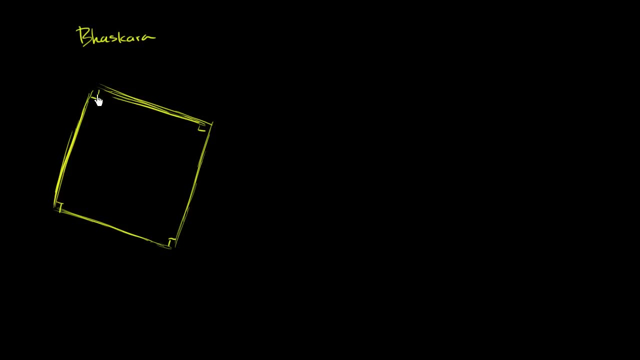 is a right angle. That's a right angle. That's a right angle. I'm assuming the lengths of all of these sides are the same, So let's just assume that they're all of length c. I'll write that in yellow. So all of the sides of this square are of length c. And now I'm. 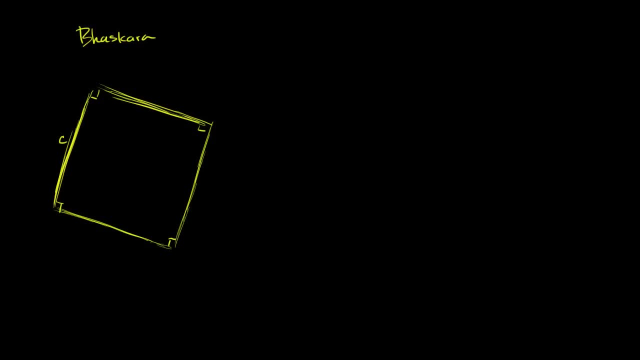 going to construct four triangles inside of this square, And the way I'm going to do it is I'm going to be dropping, So here I'm going to go straight down. I'm going to drop a little line straight down and draw a triangle that looks like this. So I'm going to go straight. 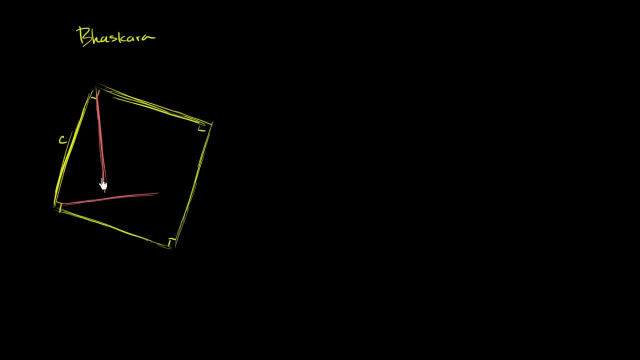 down here, Here, I'm going to go straight across. And so, since this is straight down and this is straight across, we know that this is a right angle. Then, from this vertex on our square, I'm going to go straight up. And since this is straight up and this is straight across, 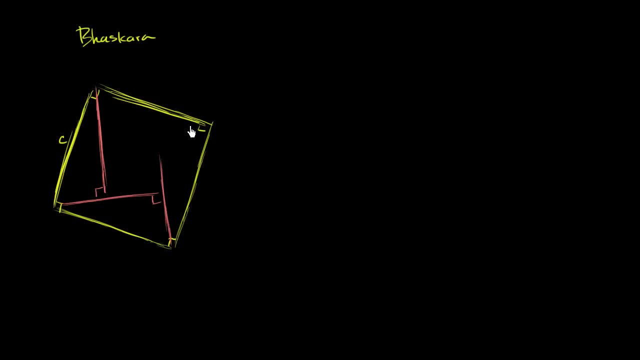 we know that this is a right angle. And then, from this vertex right over here, I'm going to go straight horizontally- I'm assuming that's what I'm doing- And so we know that this is going to be a right angle. And then we know this is going to be a right angle. 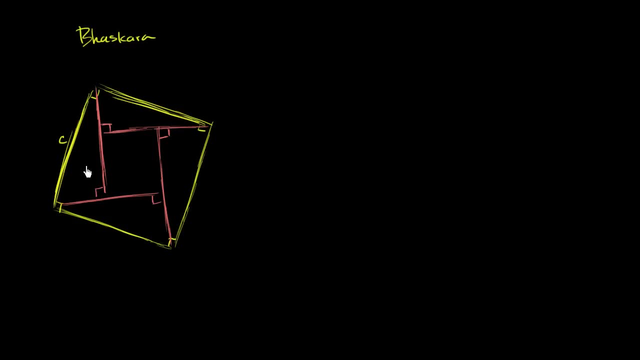 So we see that we've constructed from our square. we've constructed four right triangles And in between we have something that at minimum looks like a rectangle or possibly a square. We haven't quite proven to ourselves yet that this is a square. 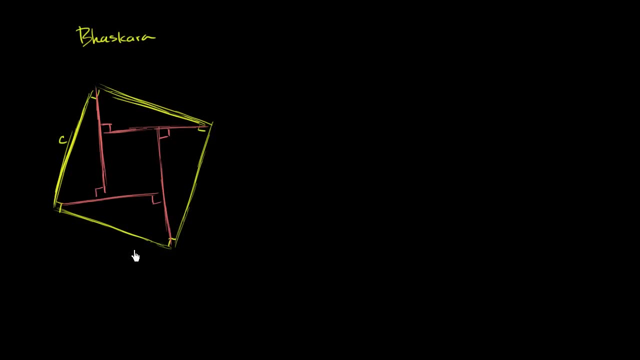 Now the next thing I want to think about is whether these triangles are congruent, So they definitely all have the same length of their hypotenuse, All of the hypo-. I don't know what the plural of hypotenuse is: hypoteni hypotenuses. 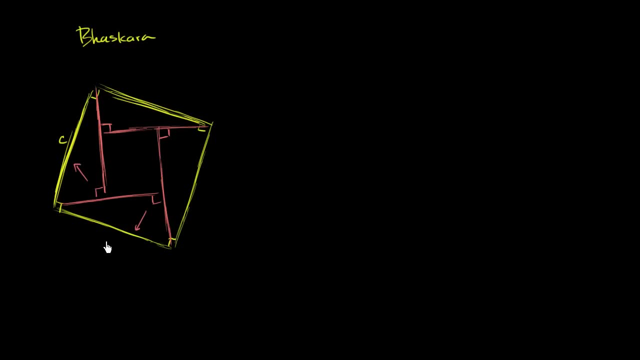 They have all length c. The side opposite, the right angle, is all ways length c. So if we can show that all the corresponding angles are the same, then we know it's congruent If you have something where all the angles are the same. 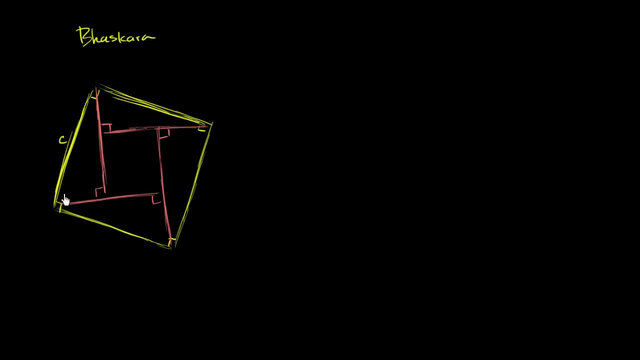 and you have a side that is also the corresponding side that's also congruent, then the whole triangles are congruent And we can show that If we assume that this angle is theta, then this angle right over here has to be 90 minus theta, because together they 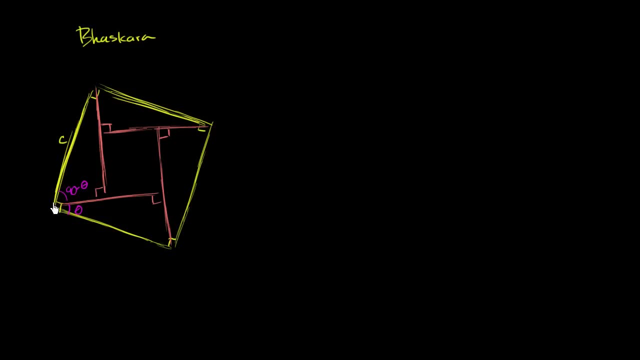 are complementary. We know that because they combine to form this angle of the square, this right angle. If this is 90 minus theta, we know this angle and this angle have to add up to 90, because we only have 90 left when we subtract. 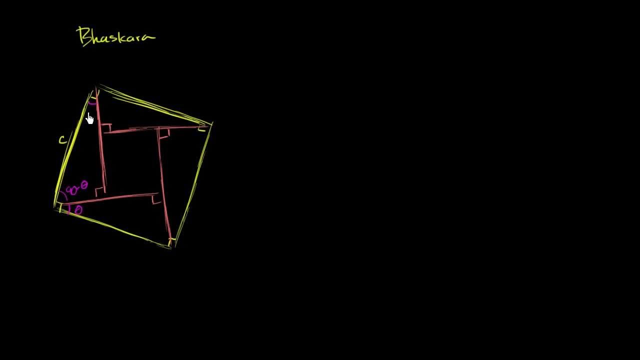 the right angle from 180.. So we know this has to be theta. And if that's theta, then that's 90 minus theta. I think you see where this is going. If that's 90 minus theta, this has to be theta. 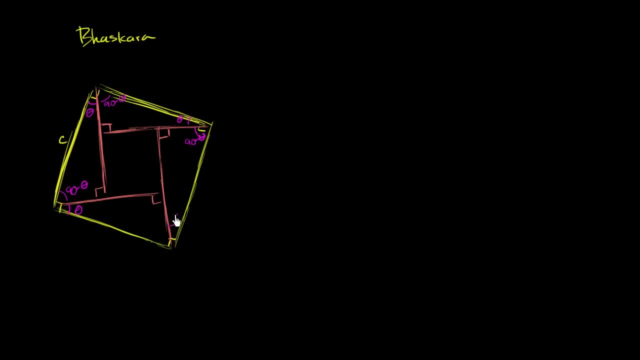 And if that's theta, then this is 90 minus theta. If this is 90 minus theta, then this is theta, And then this would have to be 90 minus theta. So we see, in all four of these triangles the three angles are theta, 90 minus theta and 90 degrees. 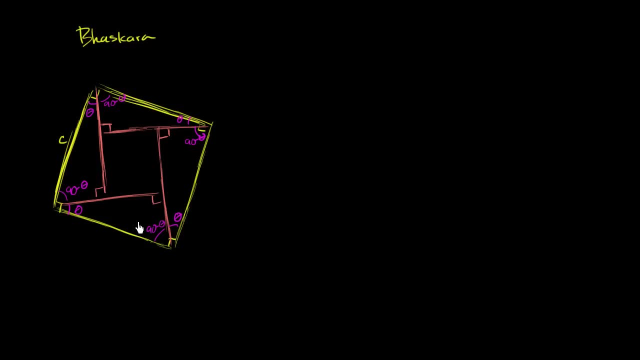 So they all have the same exact angle. So at minimum they are similar And their hypotenuses are the same. So we know that all four of these triangles are completely congruent triangles. So with that assumption, let's just assume that the longer side of these triangles 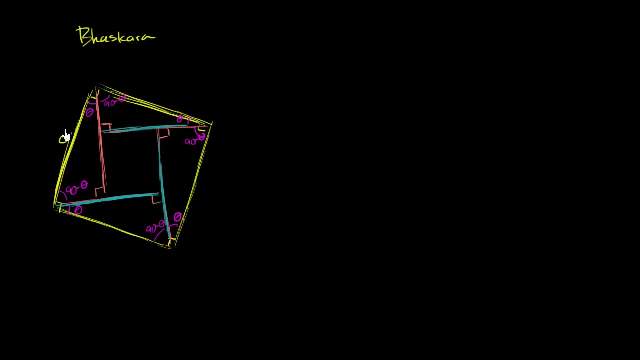 that these are of length b, So the longer side of these triangles, I'm just going to assume. So this length right over here, I'll call that lowercase b And let's assume that the shorter side. so this distance right over here, this distance right over here. 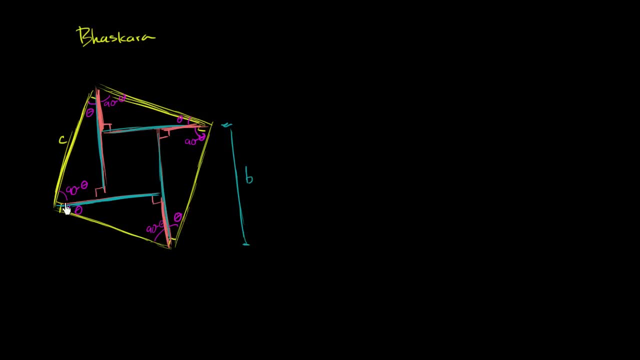 that these are all this distance right over here, that these are of length a. So if I were to say this height right over here, this height is of length, that is of length a. Now we will do something interesting. Well, first let's think about the area of the entire square. 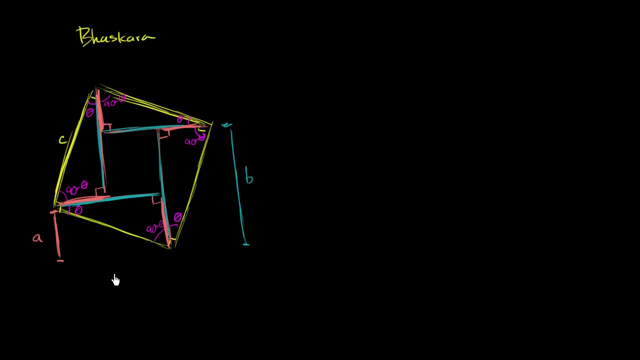 What's the area of the entire square in terms of c? Well, that's pretty straightforward: It's a c by c square. So the area, the area here, the area is equal to c squared. Now what I'm going to do is rearrange two. 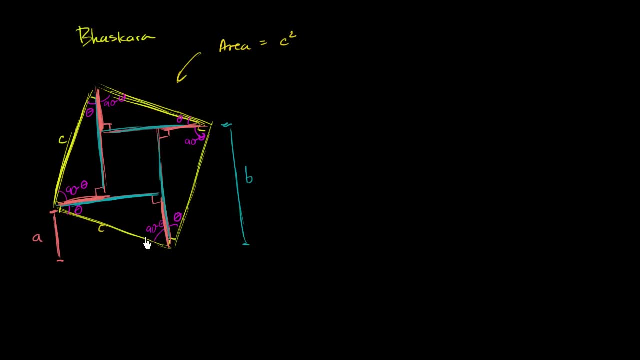 of these triangles and then come up with the area of that other figure in terms of a's and b's, And hopefully it gets us to the Pythagorean theorem, And to do that just so we don't lose our starting point, because our starting point is interesting. 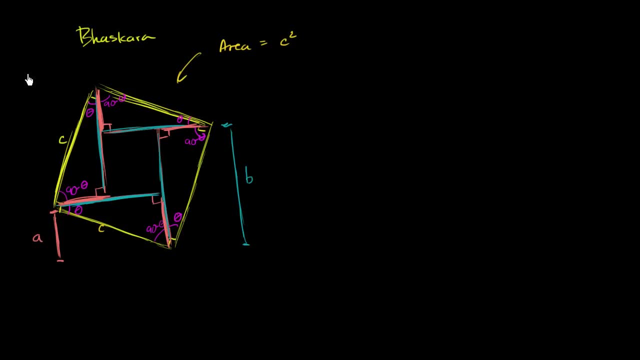 let me just copy and paste this entire thing. So I don't want it to clip off, So let me just copy and paste this Copy and paste. So this is our original diagram And what I will now do, and actually let me clear that out. 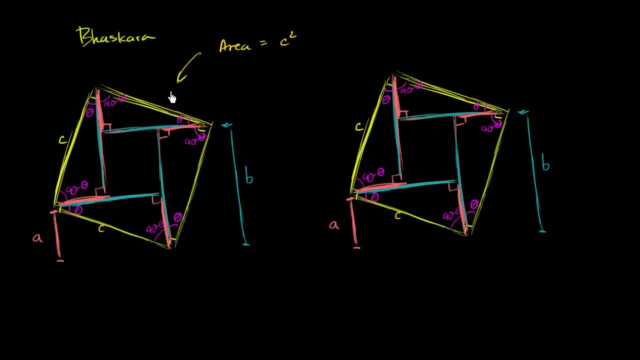 Clear. I'm now going to shift. This is the fun part. I'm going to shift this triangle here in the top left, I'm going to shift it below this triangle on the bottom right, And I'm going to attempt to do that by copying and pasting. 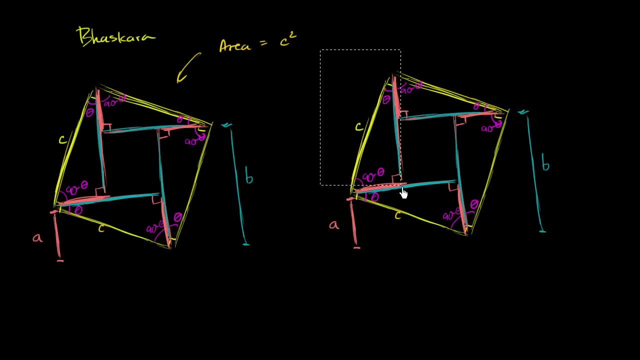 So let's see how much. well, the way I drew it, it's not that easy. Well, that might do the trick. I want to retain a little bit of this, Let's see. So let me copy, or let me actually cut it. 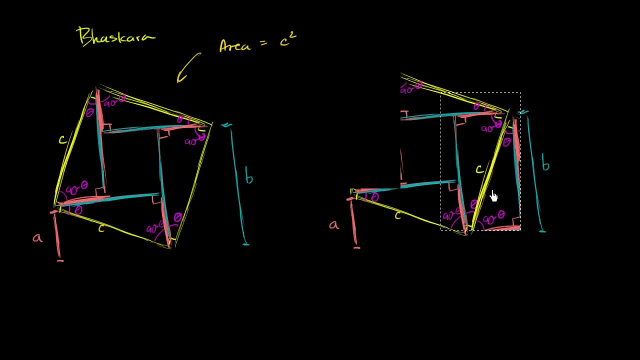 And then let me paste it So that triangle I'm going to stick right over there. Stick that right over there And let me draw in the lines that I just erased. So just to be clear, we had a line over there. 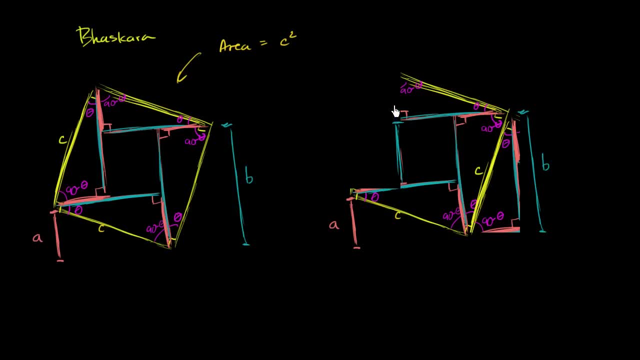 And we also had this right over here And this was straight up and down And these were straight side to side Now. So I moved this part over Over down here, So I moved that over down there, And now I'm going to move this top right triangle. 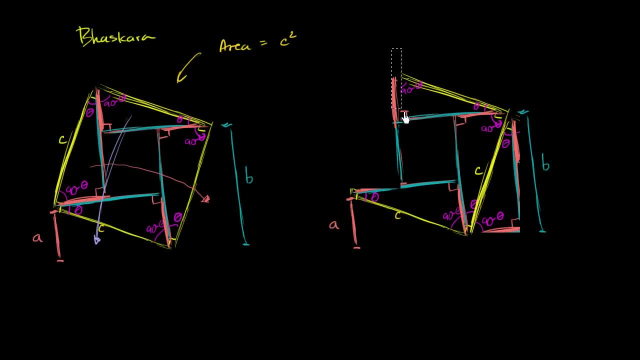 down to the bottom left. So I'm just rearranging the exact same area. So let me just capture the whole thing as best as I can. So let me cut And then let me paste, And I'm going to move it right over here. 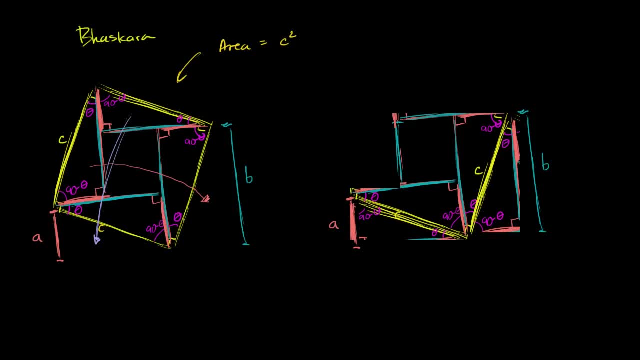 And while I went through that process I kind of lost its floor. So let me redraw the floor. So I just moved it right over here. So this thing, this triangle- let me color it in- is now right over there, And this triangle is now right over here. 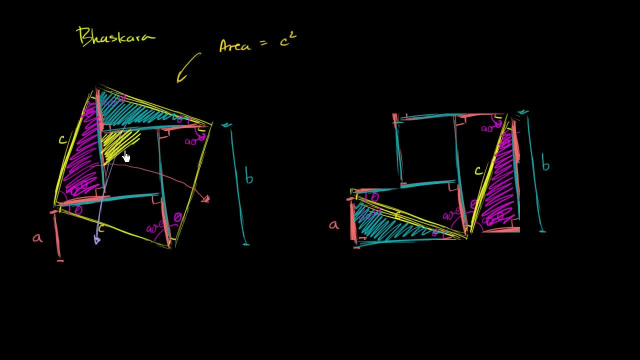 That center square And it is a square. It is now right over here, So hopefully you can appreciate how we rearranged it. Now my question for you is: how can we express the area of this new figure, which has the exact same area as the old figure? 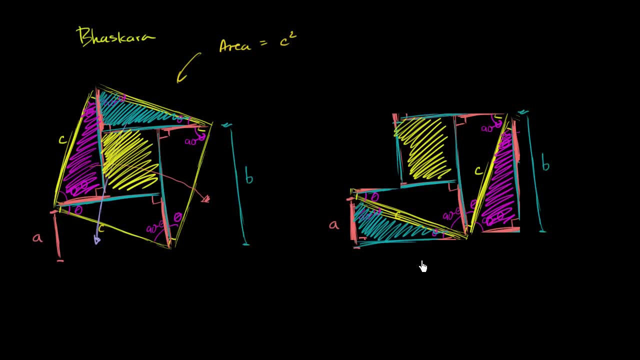 I just shifted parts of it around. How can we express this in terms of a's and b's? Well, the key insight here is to recognize the length of this bottom side. What's the length of this bottom side right over here? The length of this bottom side. 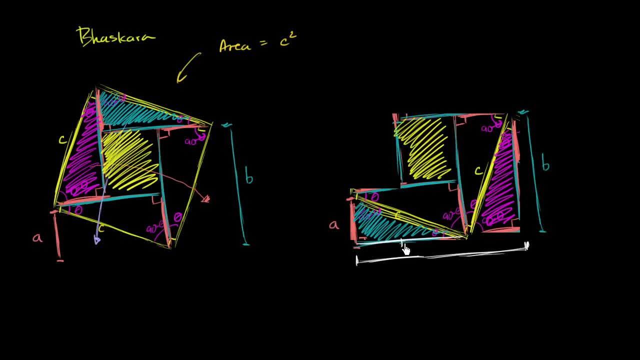 The length of this bottom side. Well, this length right over here is b, This length right over here is a. So the length of this entire bottom is a plus b. Well, that by itself is kind of interesting, But what we can realize is that this length right over here, 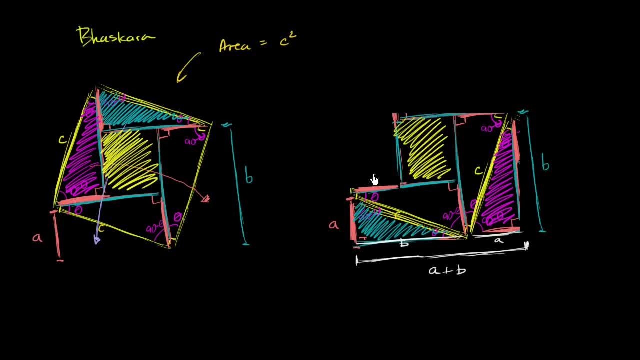 this length right over here, which is the exact same thing as this length over here, was also a, So we can construct an a by a square. So the length right over here is a by a, And so it has area a squared. 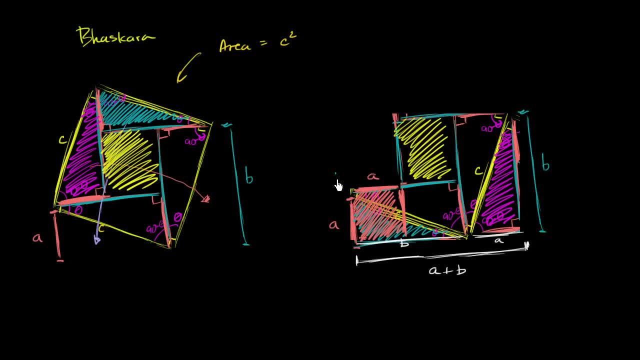 Let me do that in a color that you can actually see. So this has area of a squared, And then what's the area of what's left over? Well, if this is length a, then this is length a as well, If this entire bottom is a plus b. 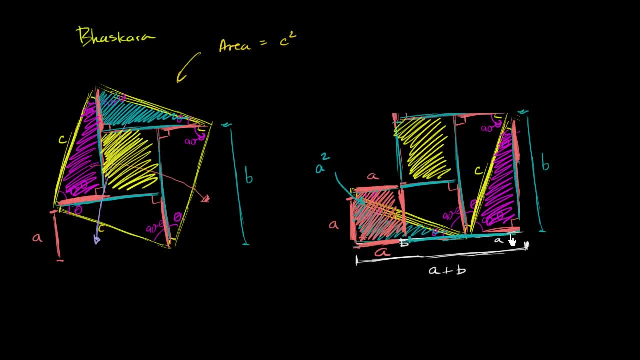 then we know that what's left over after subtracting the a out has to be b. If this whole thing is a plus b, this is a, then this right over here is b, And so the rest of this newly oriented figure, this new figure, everything that I'm shading in over here, 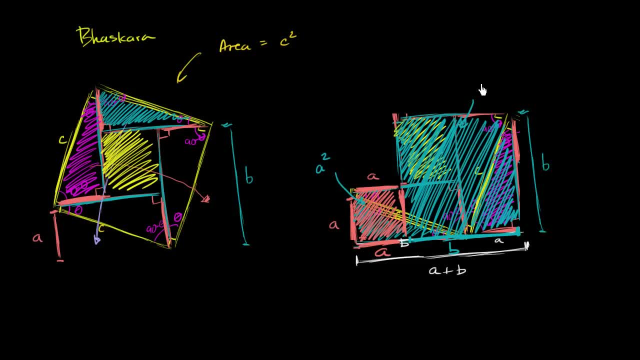 this is just a b by b squared, So the area here is b squared. So the entire area of this figure is a squared plus b squared, which, lucky for us, is equal to the area of this expressed in terms of c, because they're the exact same figure, just. 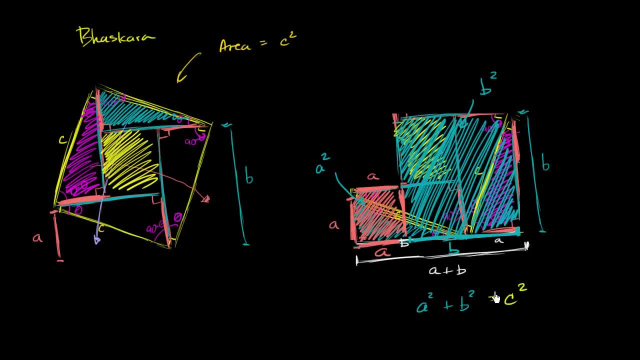 rearranged, So it's going to be equal to c squared And it all worked out And Bhaskara gave us a very cool proof of the Pythagorean theorem.